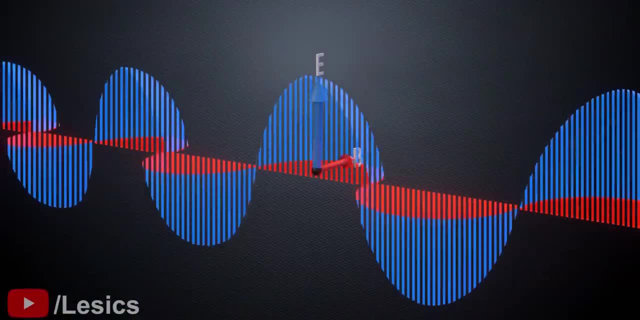 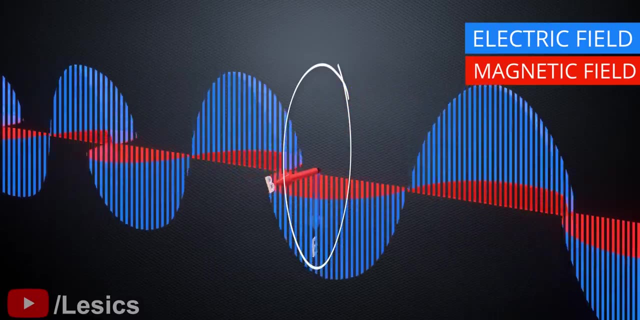 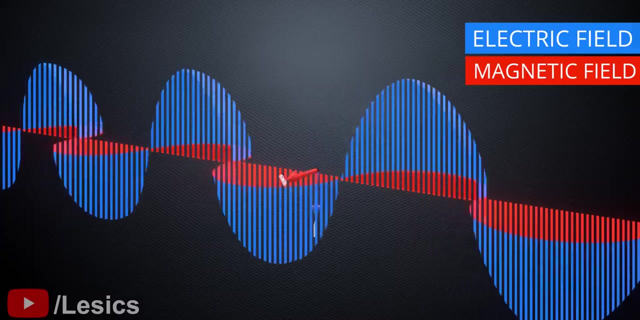 Like any other electromagnetic waves, they have oscillating electric and magnetic fields. If you track amplitude of the wave in a specific area, you can observe this oscillation. In the chocolate melting accident case, the oscillating electric field component of the electromagnetic wave is responsible for cooking the food. 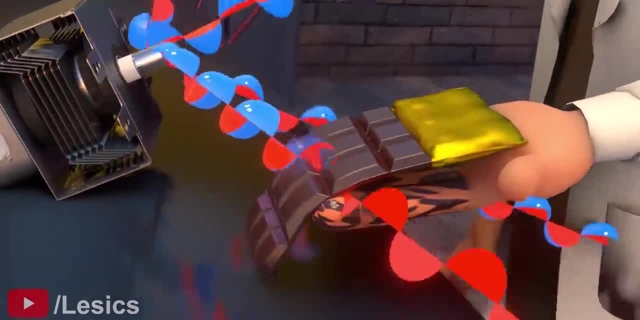 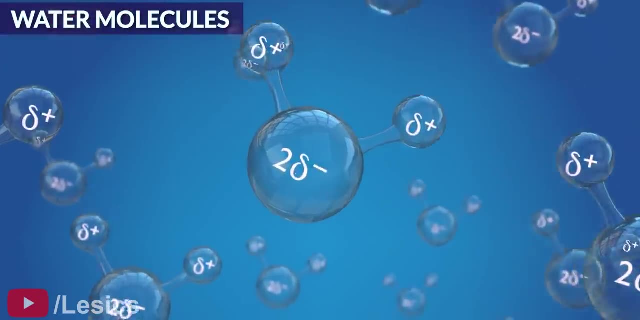 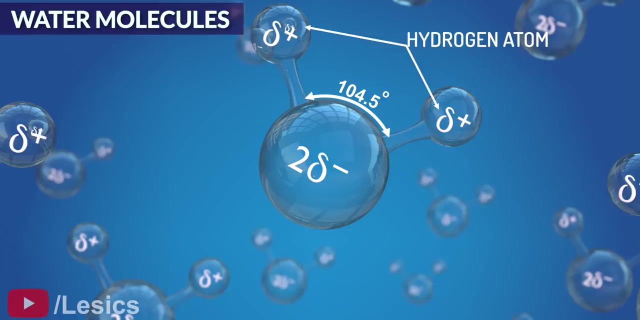 Now let's see how these oscillating electric fields cook food. Most of the food that we consume has water in it. Water is a polar molecule. The hydrogen atoms of the water molecule are placed at an angle of 104 degrees from each other, and both the hydrogen and oxygen atoms have charges. 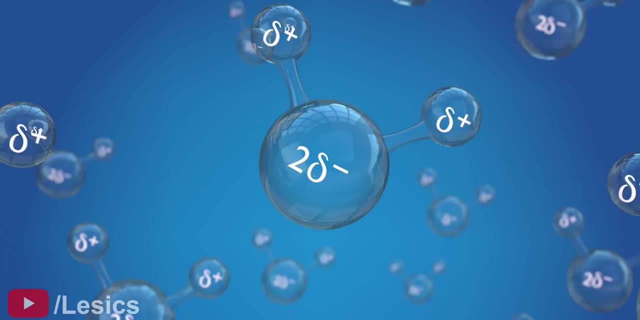 This makes the water molecule behave like a dipole. When an electric field is placed at an angle of 104 degrees from each other, the hydrogen atom is applied to the water molecule. It starts to rotate due to the torque produced on the dipole. 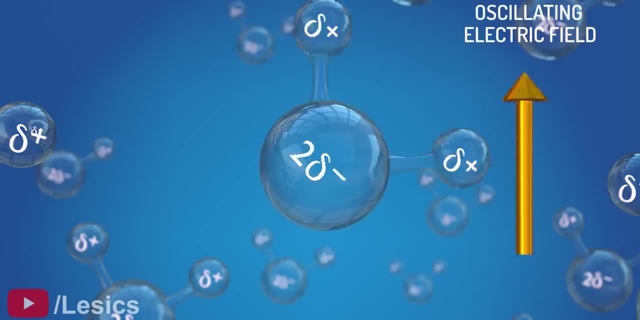 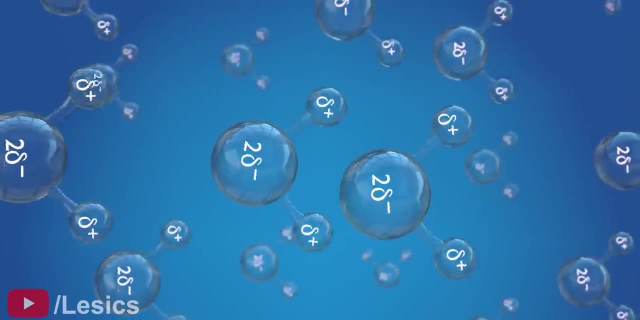 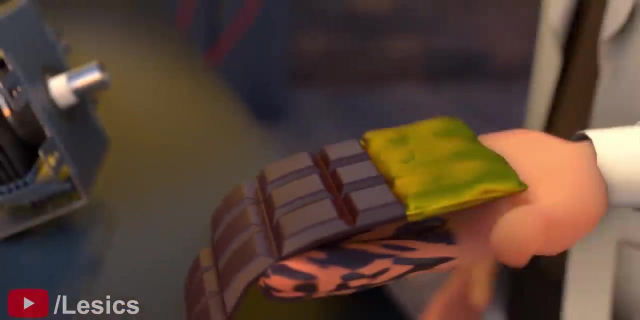 Since in electromagnetic waves the electric field oscillates continually, the water molecules will keep on oscillating. Due to this oscillating rotation, the molecules rub against each other and produce friction and heat in the food. Now let's look at how to convert this heat generation concept into a workable product. 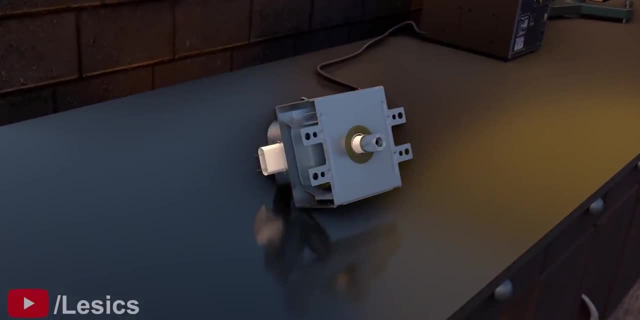 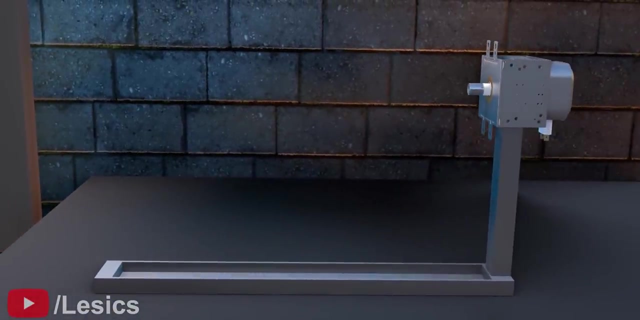 To use the electromagnetic wave's energy efficiency, we need to convert the electric field into a workable product. To use the electromagnetic wave's energy efficiently, it must be reused several times. An efficient way of achieving this is to reflect it and keep it confined in a particular area. 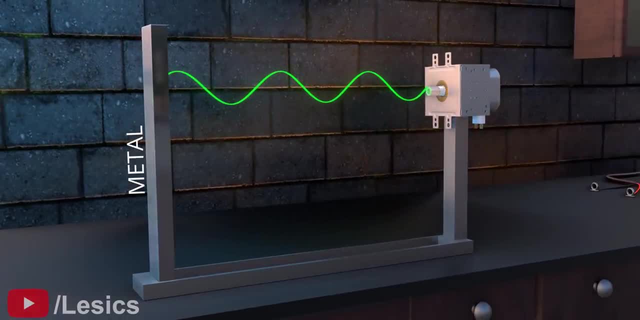 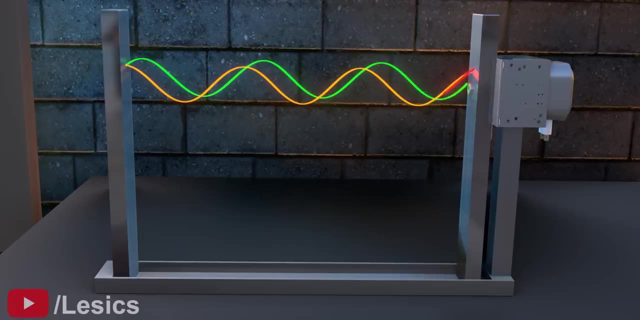 The best way of making this reflector is with the help of metal. The metallic surface causes the microwave to reflect from its surface, and if you keep one more reflector at the source side, the reflection will keep on continuing. This way, we will be able to trap the energy of electromagnetic radiation within a volume. 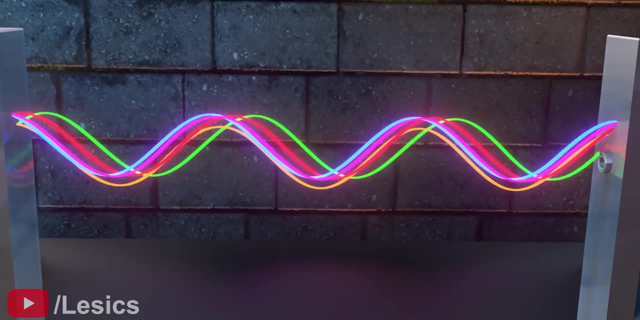 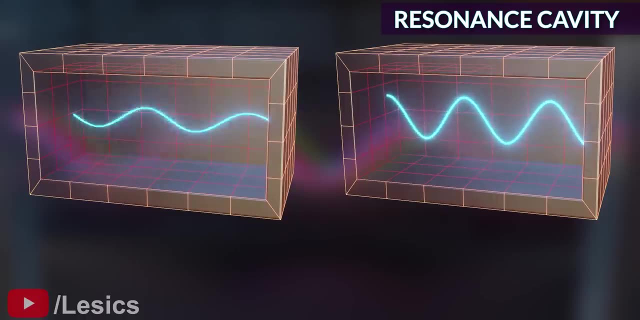 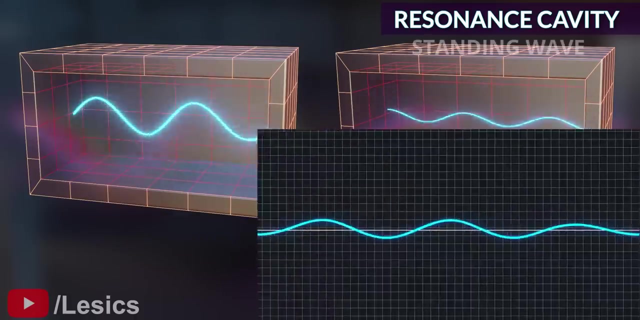 However, the most efficient way of trapping electric field energy is to use the electromagnetic wave. energy is by use of a technique called resonance cavity. This method also increases the intensity of electromagnetic waves. Let's understand the concept of resonance cavity using a simplified approach of standing. 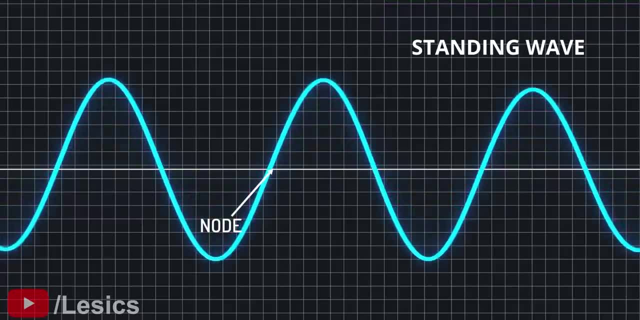 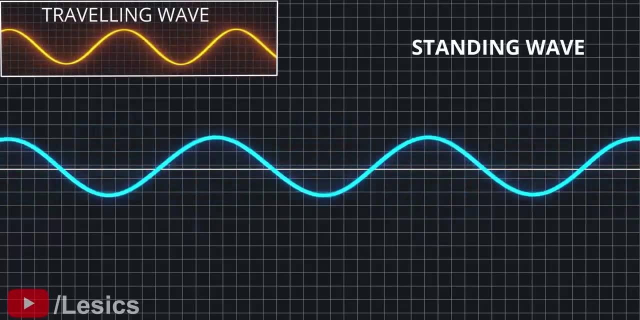 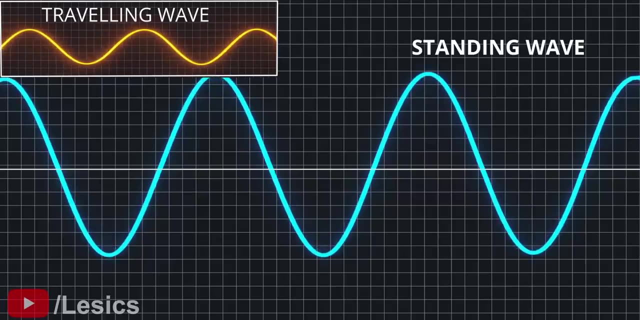 waves. A standing wave is a stationary wave that fluctuates in time but does not propagate in space. Just by observing these two wave animations you can understand how a standing wave is different from a normal traveling wave. It is formed when two waves having the same amplitude and the same frequency moving in. 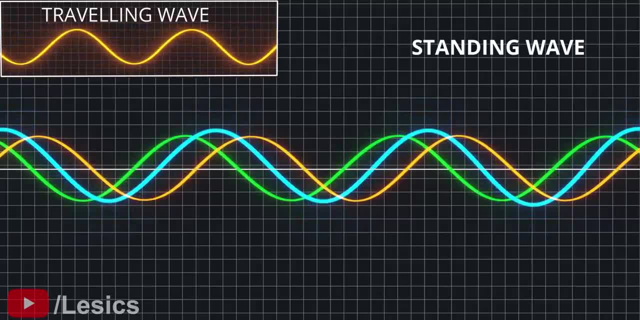 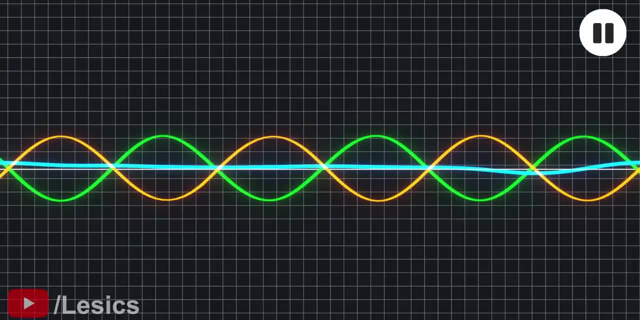 opposite directions are superimposed on each other. Please have a look at these two electromagnetic waves which are traveling in the opposite direction. Let's pause the animation here. You can see that the waves have 180 phase differences here. When you add both the electromagnetic waves, they will perfectly cancel. 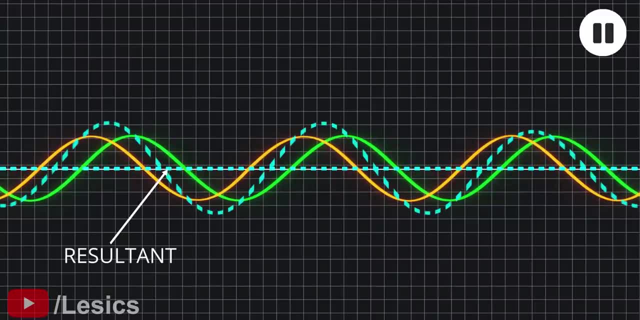 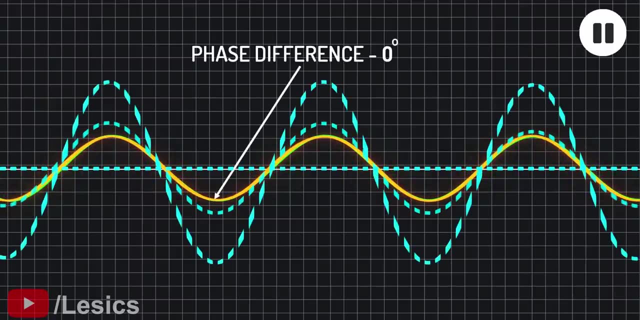 Now let's pause at this instant. The resultant is a bigger sinusoidal curve. Let's pause at one more instance. Here you are getting an even bigger sinusoidal wave as the output. By comparing the results of these three instances, it is clear that the resultant electromagnetic 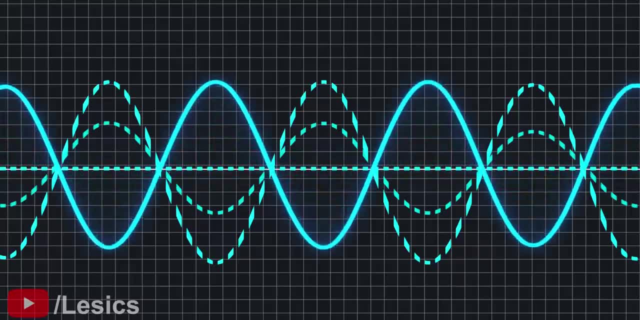 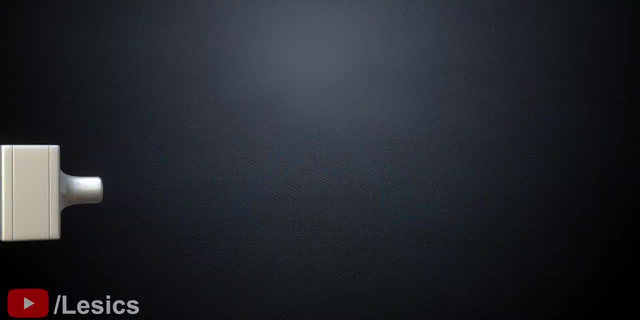 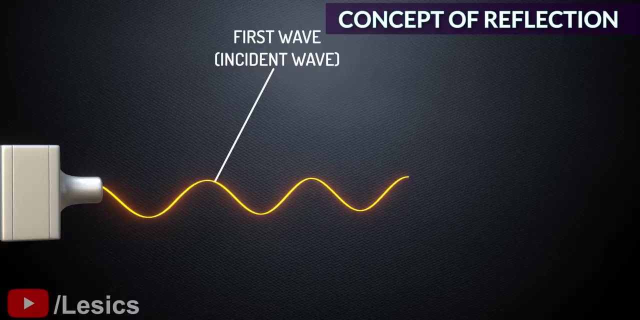 wave just oscillates in its position without traveling. Let's examine how to produce two oppositely traveling waves practically. We will get a clear solution for this if we understand how electromagnetic waves get reflected on a metal surface. We know that when a wave meets a reflector, it returns to its source. 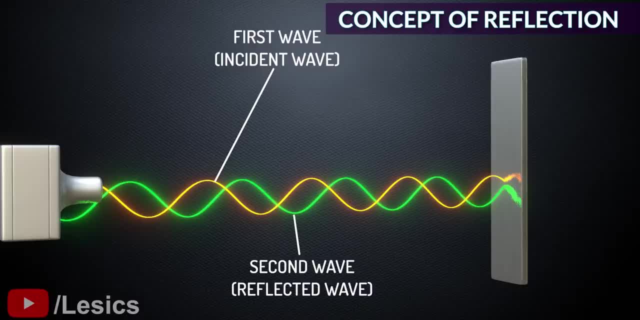 Can you spot any connection between this reflected and incident wave? The reflected wave is in fact the wave that would have traveled forward if there were no reflector. First, of course, you have to fold this imaginary part 180 degrees, as shown. 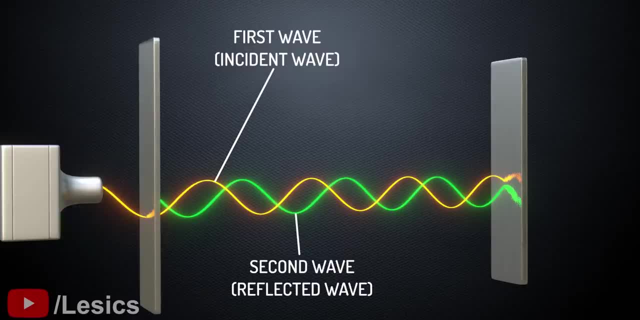 Now let's add one more reflector, this time at the side of the source. This will reflect the same way again and produce a third wave, and this process will repeat. However, if you keep the second reflector at the intersection point of the first and 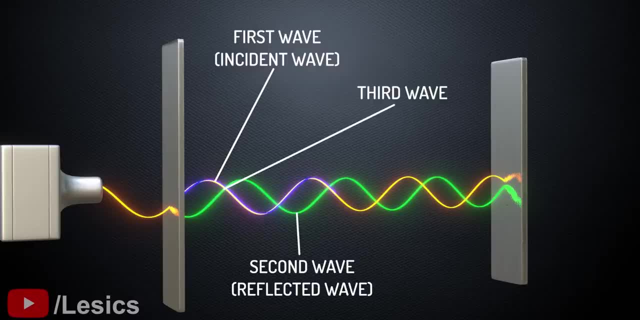 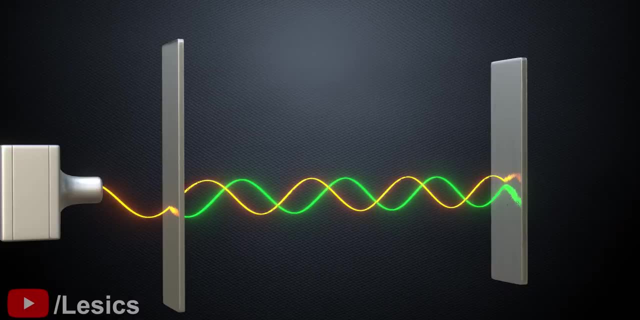 second waves. the third wave produced after the reflection will be the same as the first wave. This is a clever arrangement. When you arrange the second reflector this way, we will see only two waves traveling in opposite directions instead of many reflected waves and chaos. 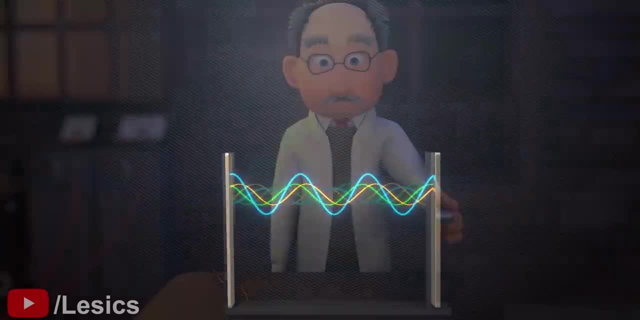 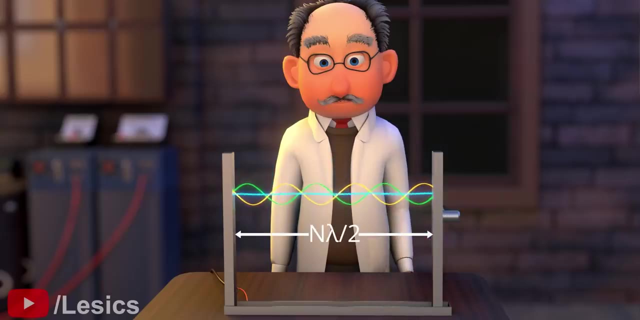 If you find out the resultant of them, it will be a negative. If you find out the resultant of them, it will be a standing wave. This is a well-known fact. The standing waves get produced when the distance between the source and reflector is an integer. 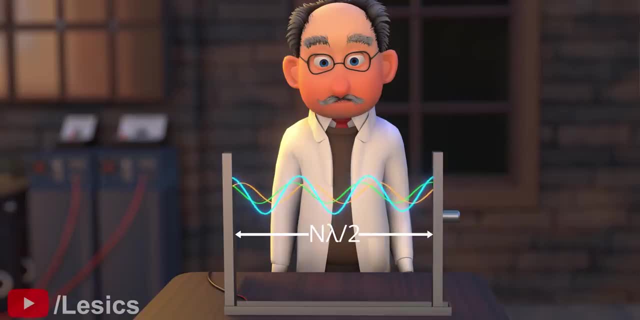 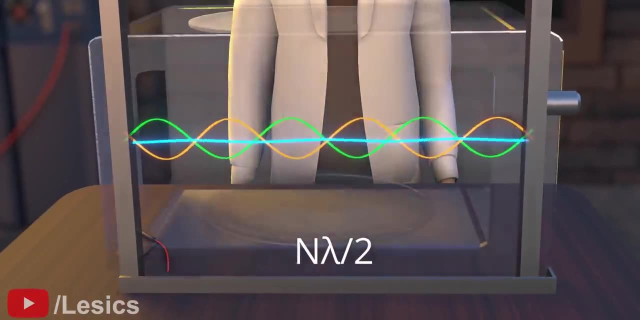 multiple of half wavelength. Thus the dimensions of the closed structure are determined by the wavelength of these waves. Now a fun fact: Just measure the cavity length of the microwave oven in your kitchen. It will be an integer multiple of this wavelength. 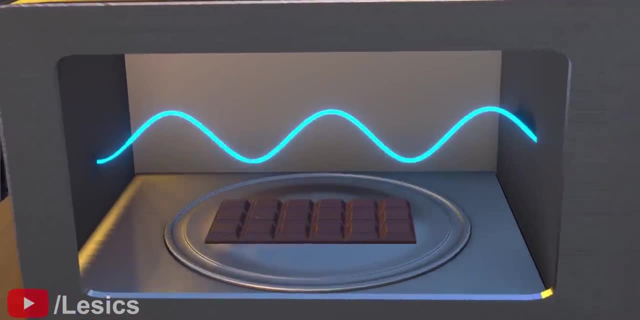 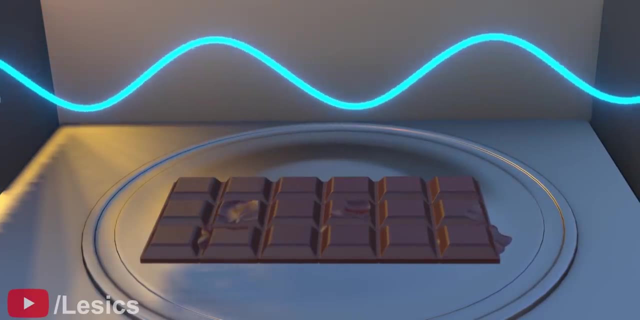 It is clear from this visual that some points of the standing wave will be equal to the distance between the source and reflector. Some points of the standing wave are at high energy intensity and some other points are at zero intensity. Due to this, there would be many spots in a microwave, some cold and others hot. 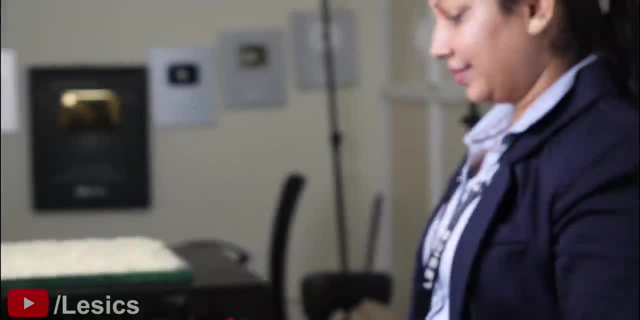 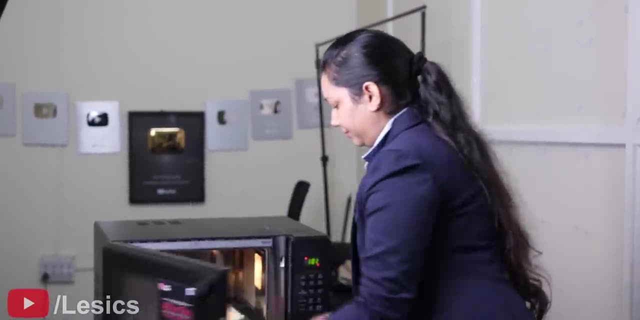 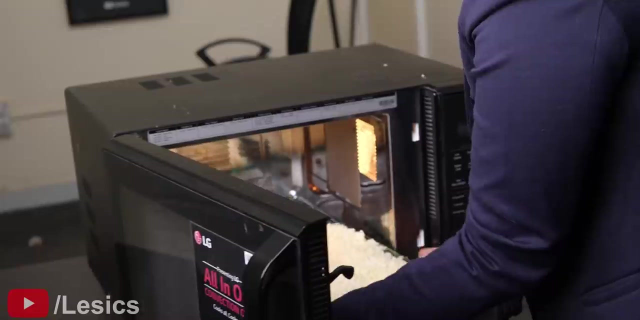 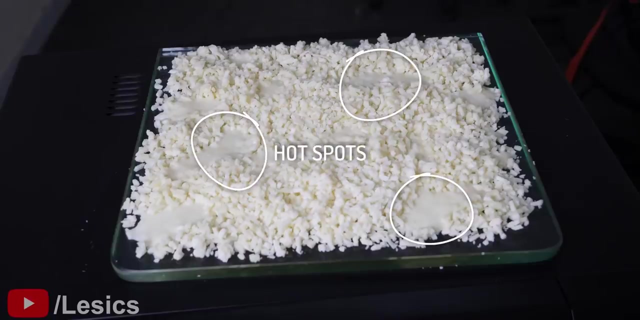 Using cheese. you can demonstrate these cold and hot spots of your kitchen's microwave oven. Just keep the shredded cheese inside your microwave oven for one minute. What you see after one minute is the cheese surface with a few hot spots. The presence of such hot spots causes a microwave to cook food unevenly. 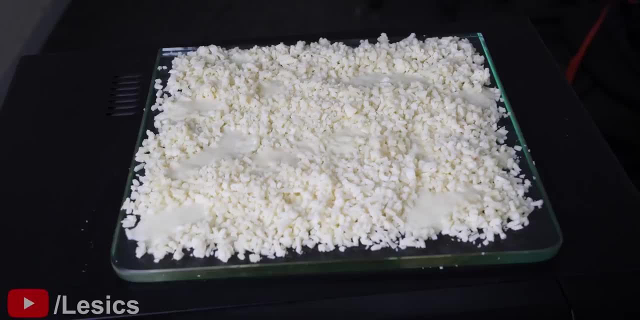 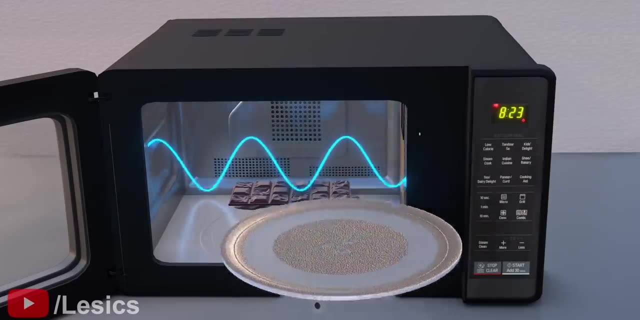 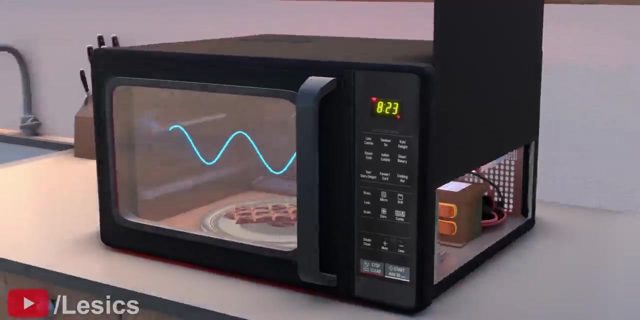 In short, the cavity resonance technique we use to trap the microwaves more efficiently has led to creation of cold and hot spots. To overcome this problem, nowadays a microwave consists of a rotating plate which helps the food cook evenly. The component responsible for producing heat is the microwave. 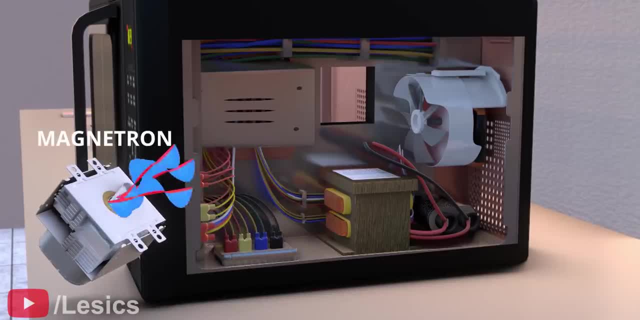 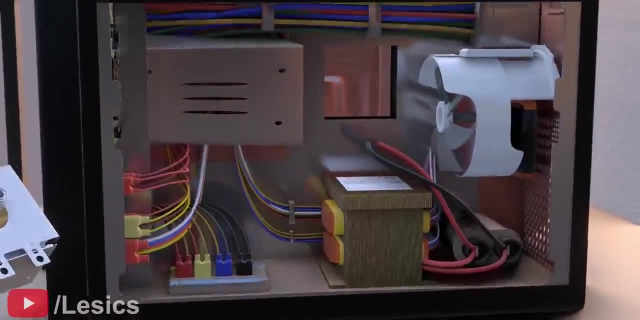 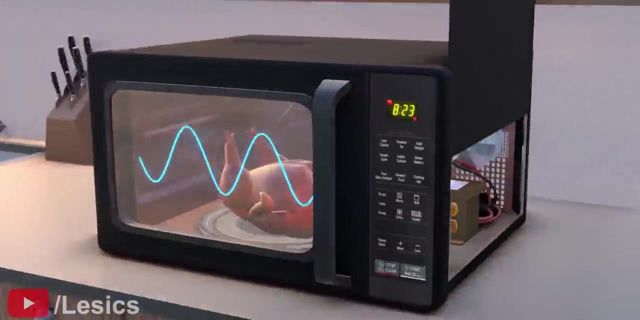 The component responsible for producing microwaves is known as a magnetron. A magnetron emits microwaves in all directions. To confine the wave to propagate in one dimension, the magnetron is attached to the waveguide. From the waveguide the waves come into the cooking chamber to heat food. 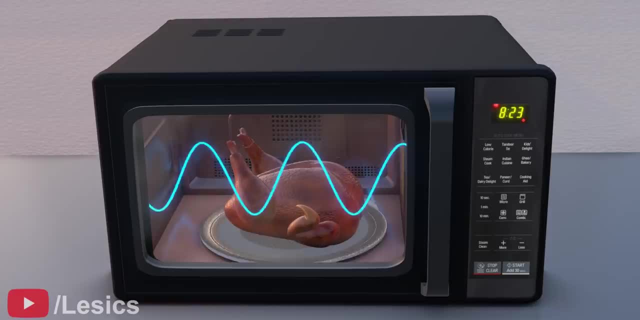 Another question that has to be answered is whether microwaves are the only electromagnetic waves capable of heating food, or if there are any other waves that could accomplish the same result. Any electromagnetic waves have the capability to heat food, but they come with certain limitations. 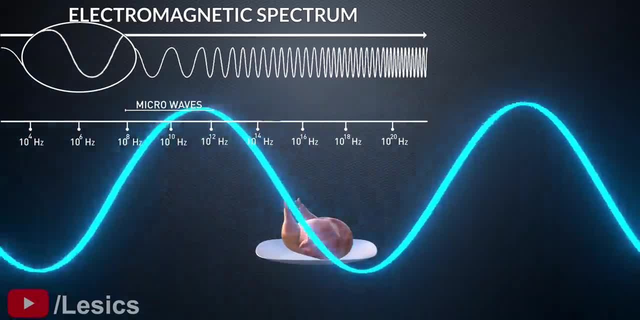 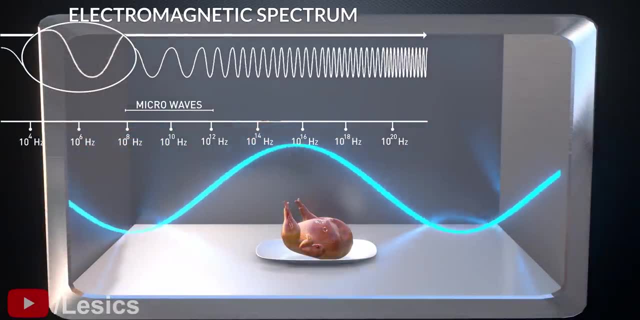 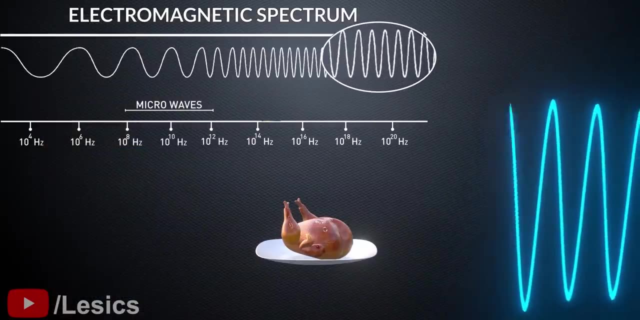 Waves with long wavelengths can easily pass through our food, so that they won't be able to transfer much energy to it. Additionally, to get standing wave, large devices would be required. Shorter wavelength waves are absorbed more rapidly on the outer surface of the food. 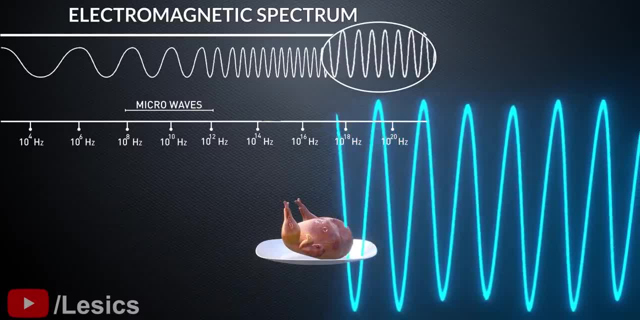 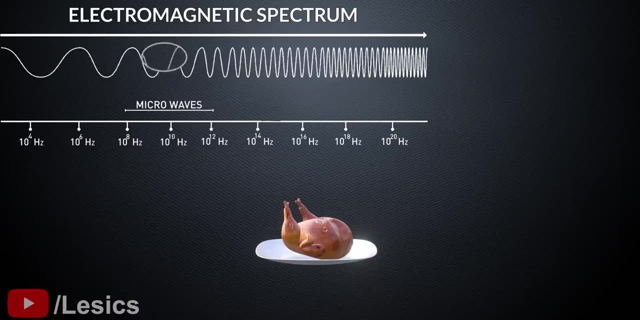 so they do not penetrate far enough down to cook it evenly. What's the difference? If we want to cook deeply, we have to switch to a very high power source that would be unfeasible In the microwave range. the suitable frequency for all practical purposes and which did.